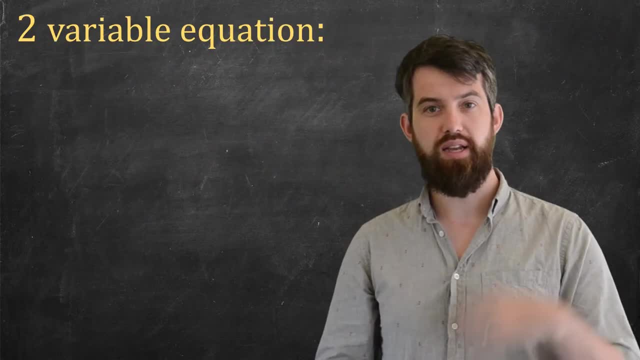 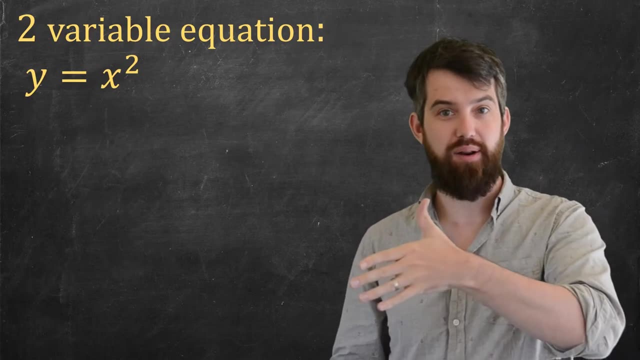 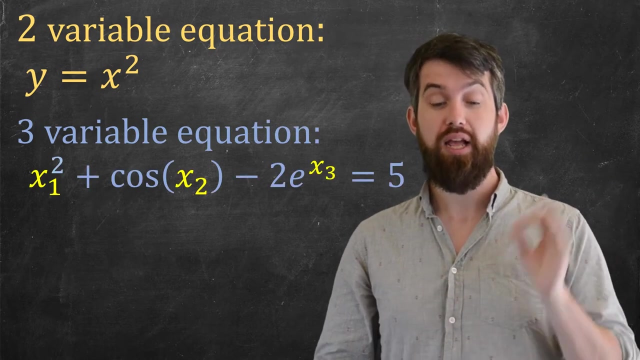 Consider the equation y equals x squared. What this does is it has two different variables, y and x, and it expresses some relation between them, And I can imagine an equation that had more variables than just the two here, For example, the equation x1 squared plus cos of x2, minus 2e to the power of. 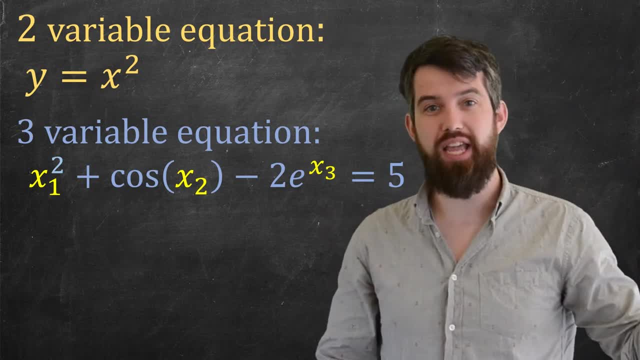 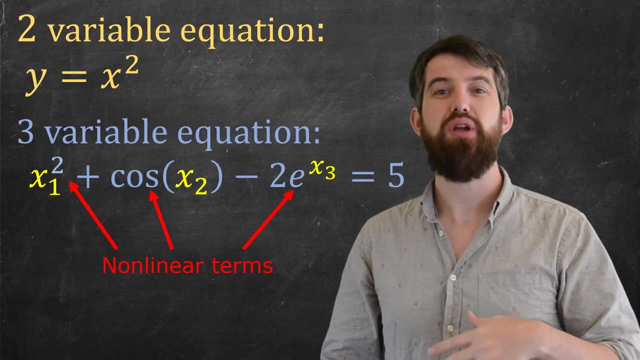 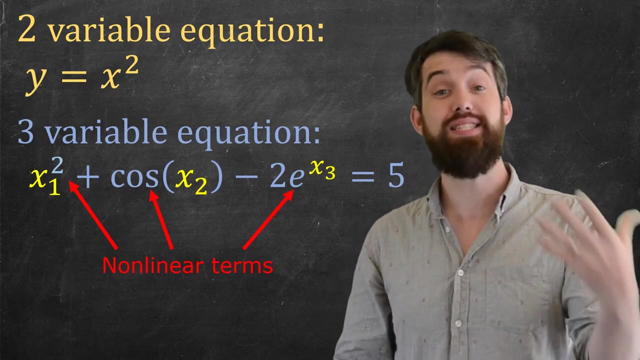 x3 equals 5.. That's just some messy equation in three different variables: x1, x2, and x3.. Now these kinds of so-called non-linear equations, equations with exponentials and signs and squares in them, they're very complicated. You can study them, but the study of them, 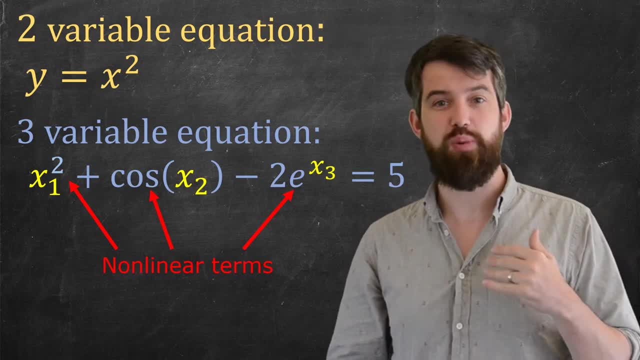 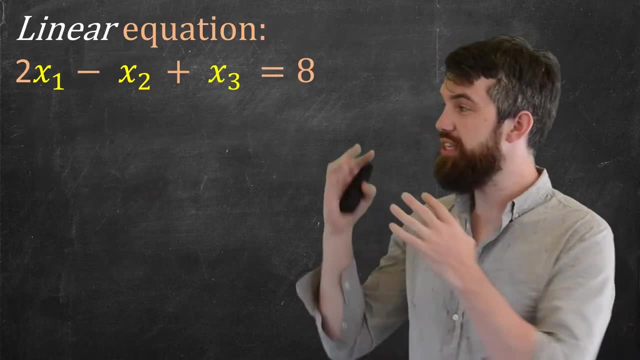 is very messy And in our course in linear algebra we're going to look at equations that have multiple variables, but we're going to restrict ourselves to a specific type. What we're going to study in this course are these linear equations. 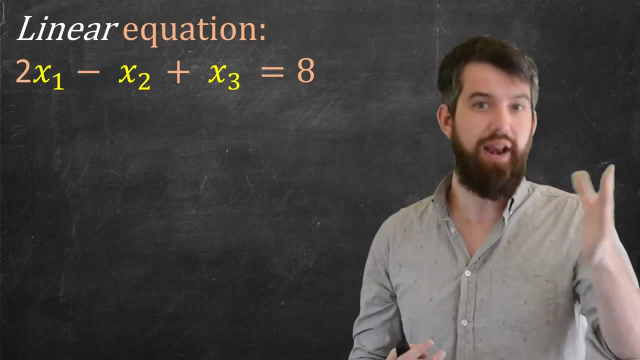 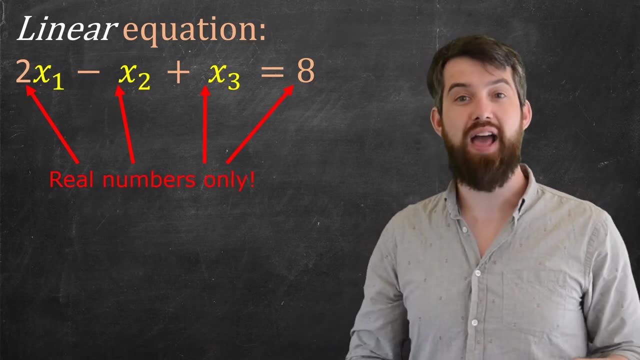 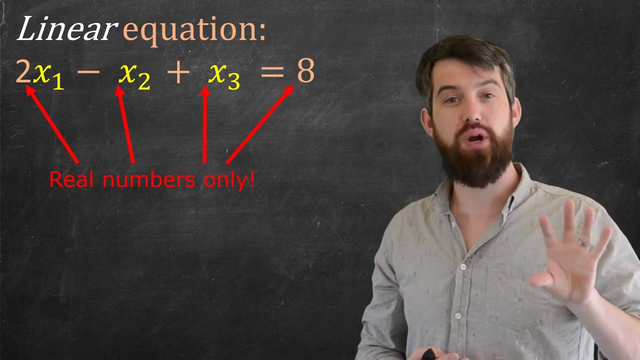 Equations where every variable, like x1,, x2, x3, it just occurs to the power of 1.. I might multiply those variables by various coefficients, numbers like 2 and minus 1, and 1 and 8, but any variable it's only going to occur to the power of exponent 1.. 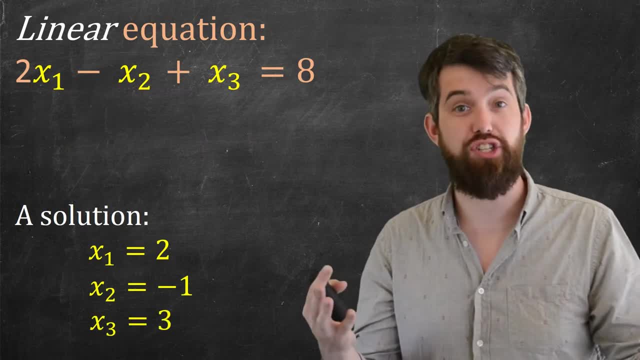 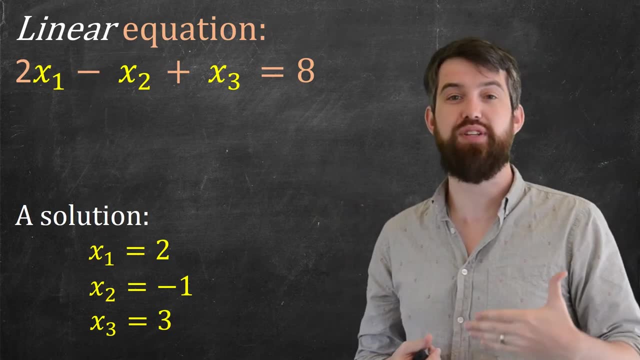 Then a solution to a linear equation is just me telling you what the x1,, the x2, and the x3 values are going to be If I specify some list of numbers. for example here: 2 times 2 is 4, minus. minus 1 is 5, plus. 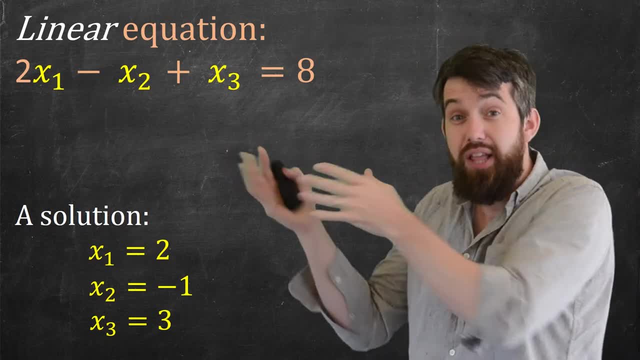 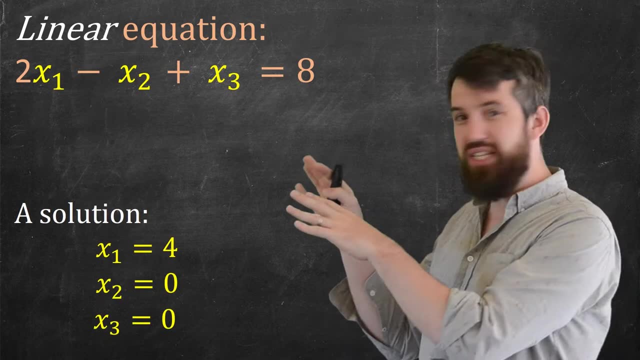 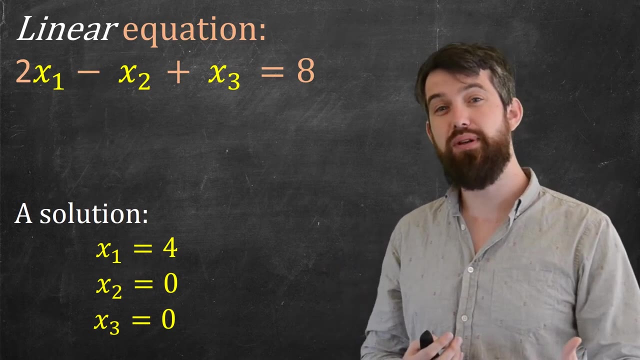 3 is 8, if I plug those numbers into the equation then it does indeed satisfy it. So that is a solution to a linear equation, And one thing to note is that often these linear systems have multiple different solutions. For example, x1 is 4,, x2 is 0, and x3 is 0 is also a solution That also satisfies this. 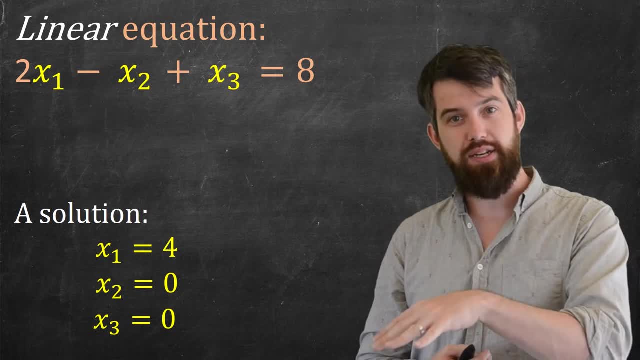 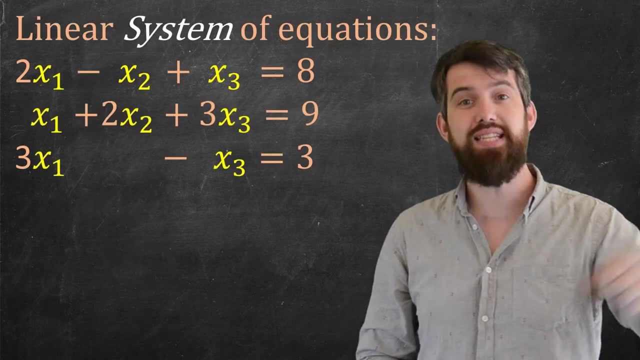 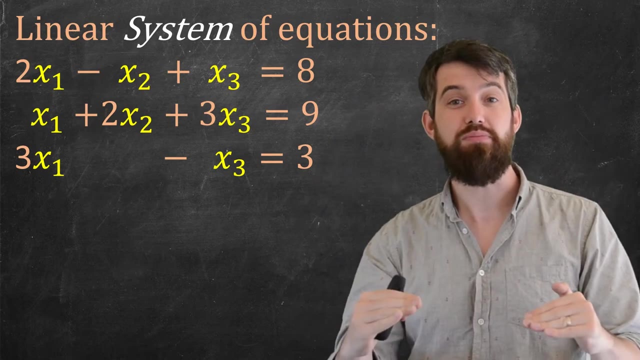 equation: 2 times 4 is 8, plus 0 plus 0 is equal to 8.. Okay, so that was linear equations, which is nice, but now let's upgrade. Let's look at linear systems of equations, And in a linear system of equations, what we're going to have is multiple lines of linear 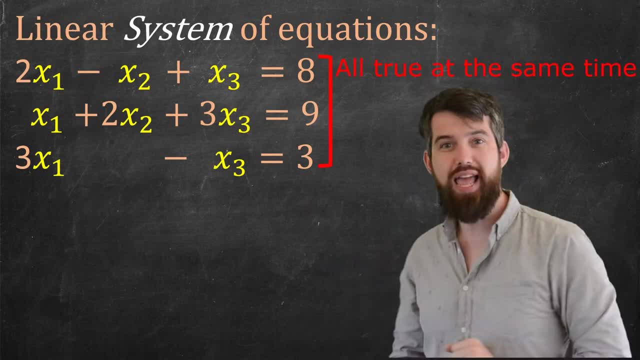 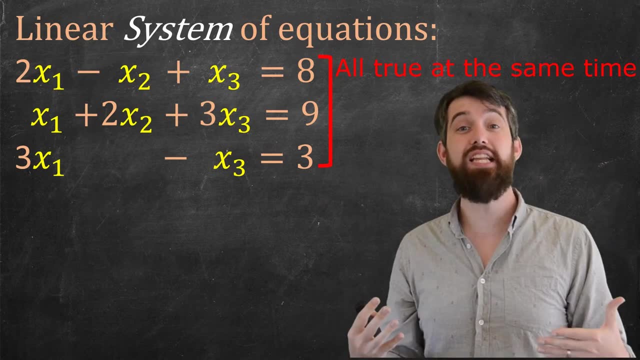 equations And the key point is that all of these equations that I have, they're true at the same time. A solution to the system of all three equations must solve each equation individually. So, for example, if we look at that, 2 minus 1,. 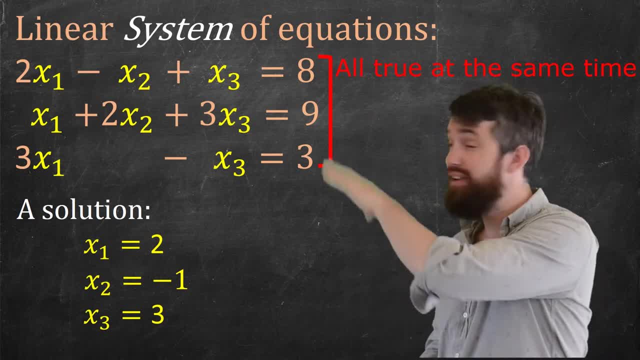 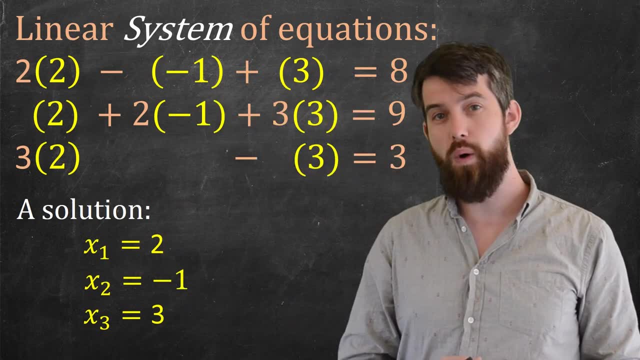 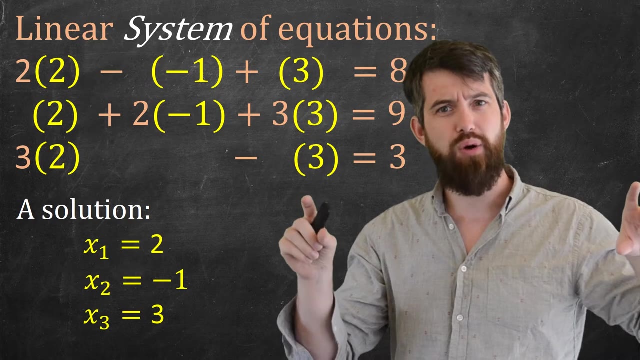 3,. well, if I plug that in, everywhere I have an x1,, an x2, or an x3, indeed it does satisfy, And we can plug it in and check that all of those numbers are indeed equalities. But I do want to note something here. Remember the solution: 4, 0, 0, just to the top row. 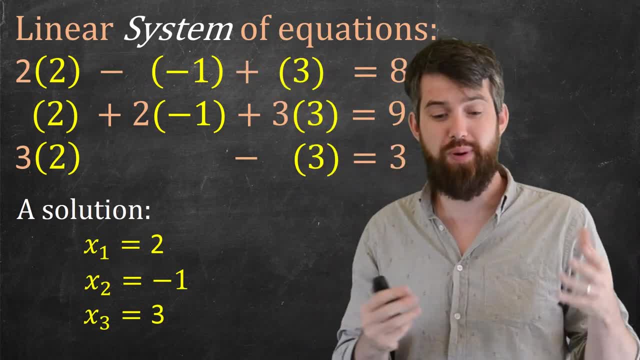 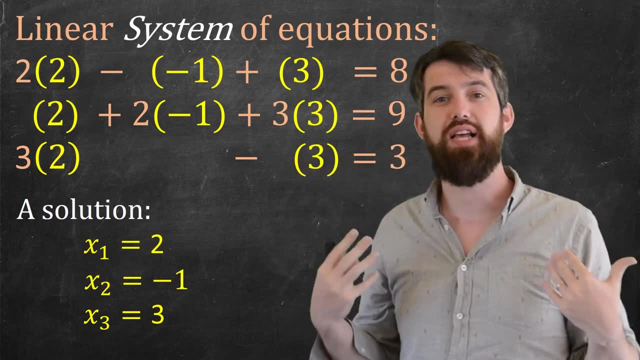 That still is a solution to the top row. 4, 0, 0 is a solution to the top row, but it is not a solution to the bottom row any longer. It is not the case that every solution to an individual equation solves the entire solution. 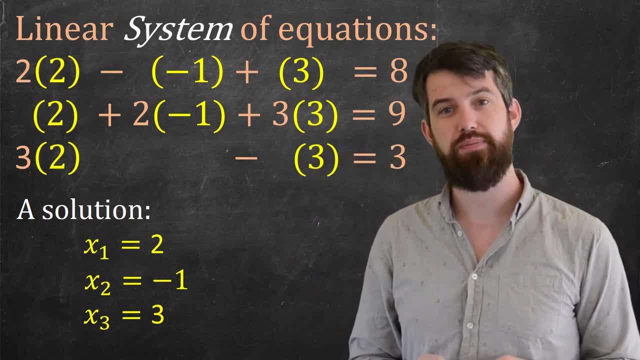 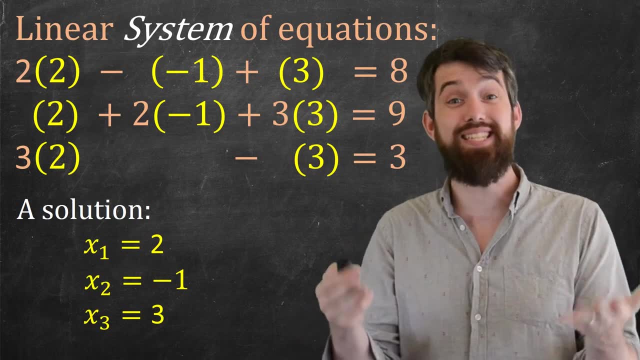 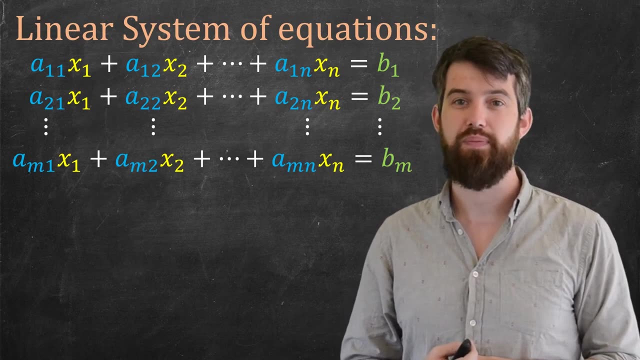 It has to solve all three equations. Now, linear systems can get big and complicated. There can be many different rows, there can be many different variables, so we want a systematic way to express it, And our systematic way is this. It's using something called AIJ notation. 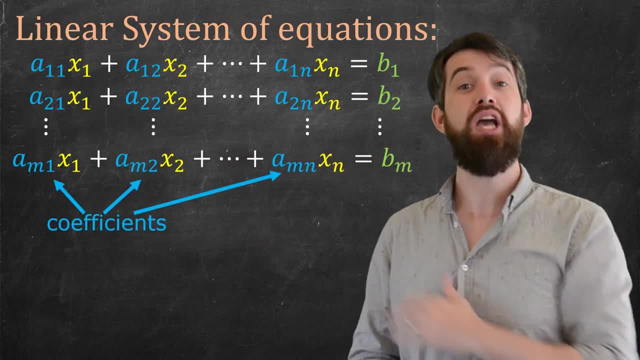 So what I have? all of the blue, all of these are my coefficients. They're just some number like 3 and 7 and 0 and minus 1 and pi and whatever you might like, And then the x1 down to the xn. that's the same thing. 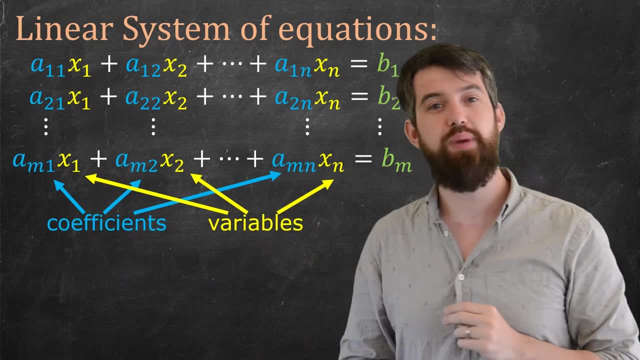 And then the x1 down to the xn. that's the same thing. And then the x1 down to the xn. that's the same thing. And then the x1 down to the xn. those are going to be my variables. That's the thing. 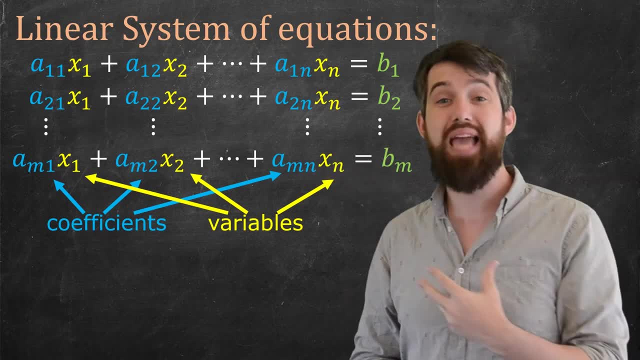 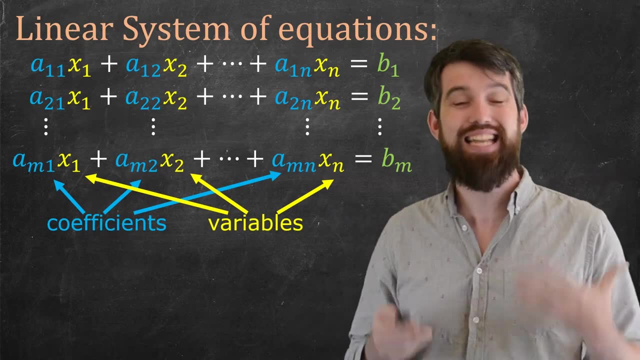 I'm trying to solve for. And then the b1 down to the bm. these are also just numbers, but because they're not associated to a variable, they don't have a variable attached to them. I'm going to call them a bit of a different name. I'll call the bs constants and I'll 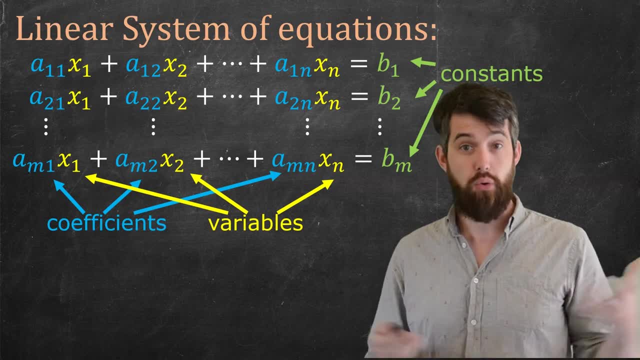 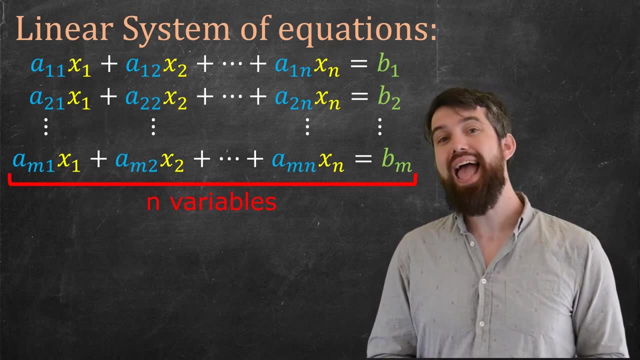 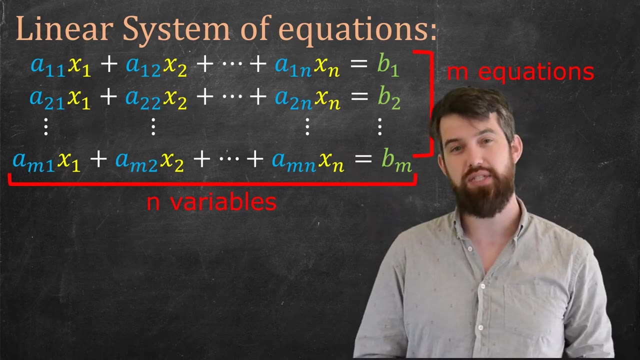 call the AIJs coefficients. So what do I have in this system? I have n different variables, my x1 down to my xn, and I have m different variables. So I have n different variables. So I have n different equations, b1 down to bm, enumerating the different rows in my linear system. 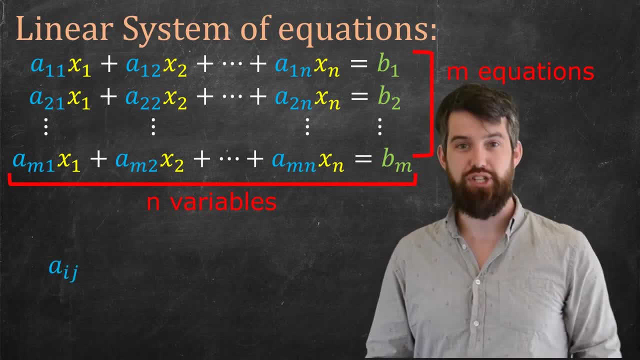 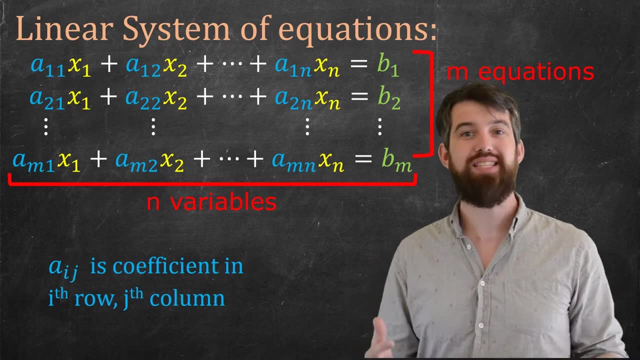 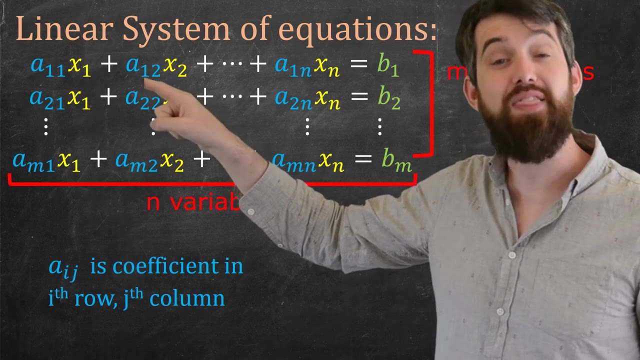 And then the way to refer to the AIJ notation is that AIJ represents the i'th row and the j'th column. So, for example, a12, well, that's going to be this one right here. It's the first row and the second column when I reference a12..